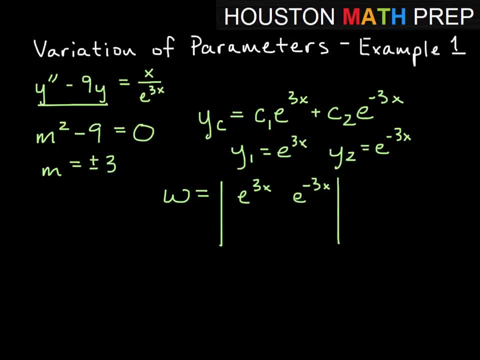 minus 3x And their derivatives in the second row. so 3e to the 3x and derivative of e to the negative 3x would be negative 3e to the minus 3x And that's going to equal this diagonal minus this. 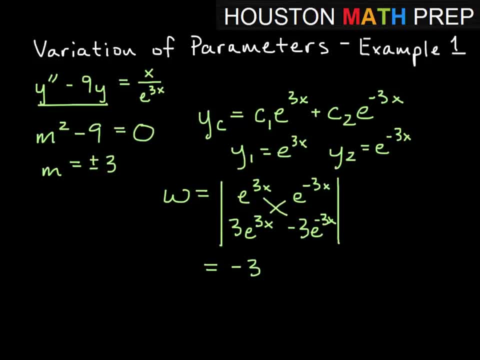 diagonal. So we'll get negative 3e to the 3x e to the minus 3x, minus 3e to the 3x e to the minus 3x. So you'll notice e to the 3x e to the minus 3x. multiplying those together we'll get 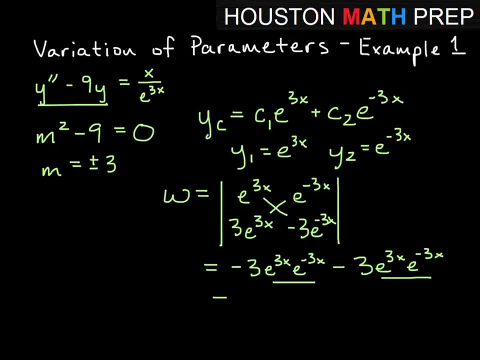 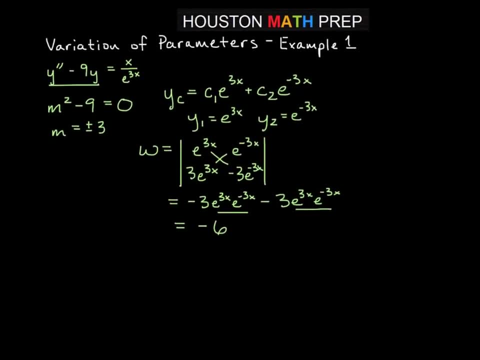 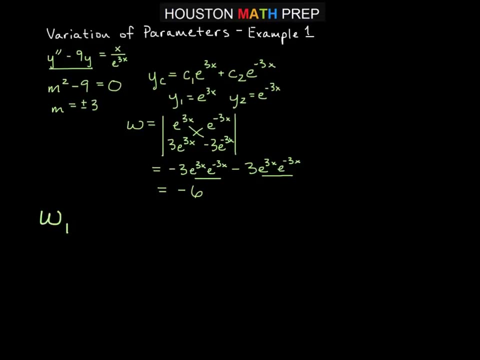 e to the 0. So we'll get negative 3 minus 3.. So, our Ronskian, there will be negative 6.. And now we need to continue by finding w1 and w2 as well. Remember, for w1, the 1 telling us to take out the first column of our original Ronskian and 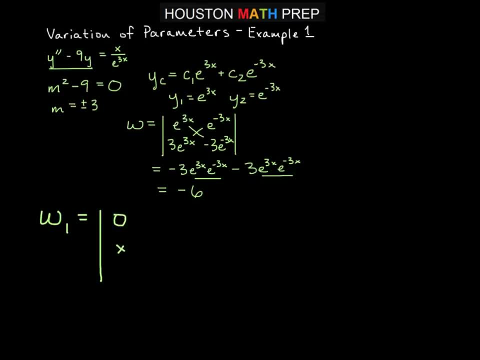 replace it with all zeros, except for the last entry being equal to g sub x. So we'll have zero and then e or sorry, x over e to the 3x which is our g of x up there. So we'll leave the second column alone: e to the minus 3x, negative 3e to the minus 3x, If we do our. 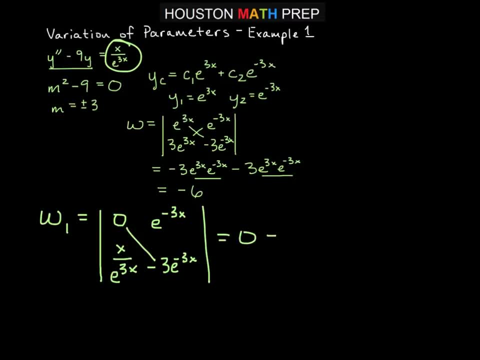 determinant, the first term will be 0 there. minus x over e to the 3x times e to the minus 3x, Minus x over e to the minus 3x, Minus x over e to the minus 3x times e to the minus 3x, And so that will then give us 0 there. 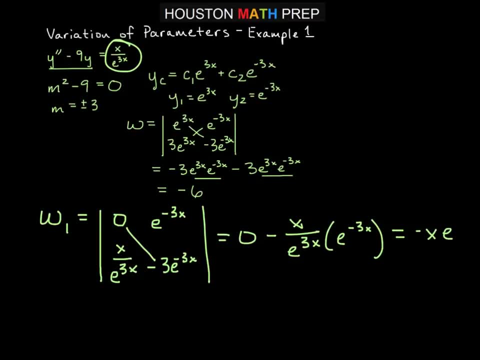 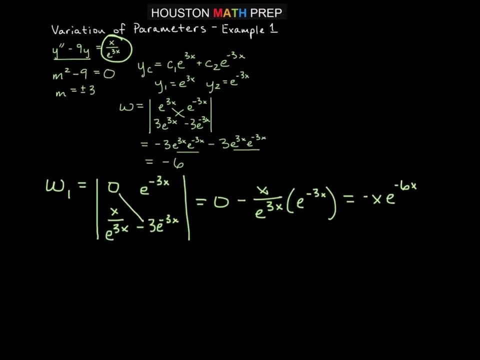 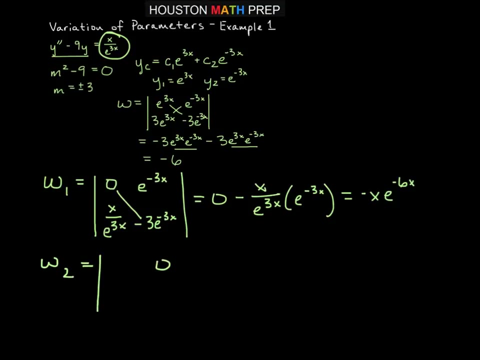 will then give us their negative x. e to the minus 6x would be the simpler way to write that. and now we also need w2. so w2 then that means we replace 0 and g sub x in the second column. so 0 and x. 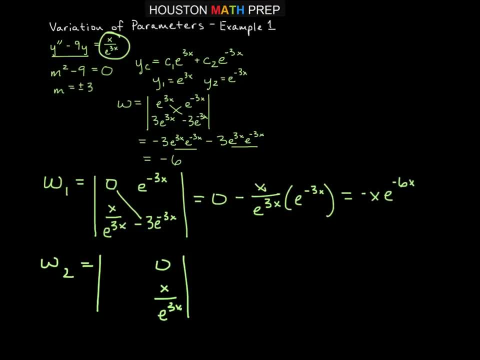 over e to the 3x, go in column 2, and then we'll leave column 1 alone from the original, which is e to the 3x and 3e to the 3x. and now doing derivative there, we'll get x over e to the 3x times e to the 3x, minus. when we do that diagonal that'll be 0. 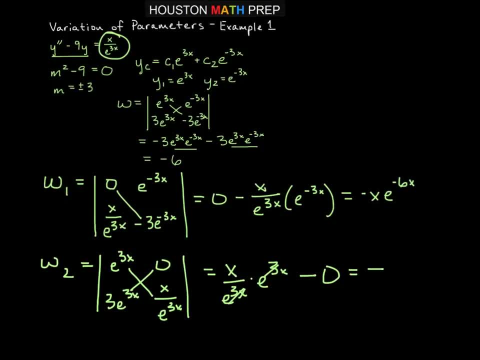 so these will reduce and that will give us x for w2. okay, so now, based on everything that we've written in the first column, we're going to do a piece of, should be able to take this and put in the two wire to appeared in this and what this equals to in the second column. 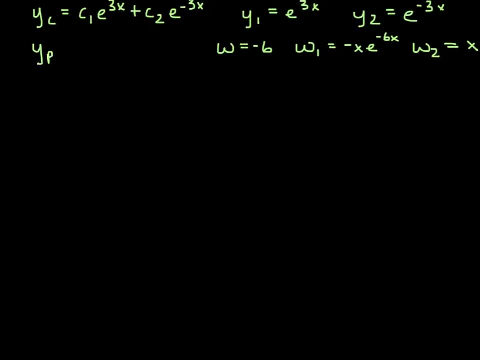 we have. so we're trying to develop the particular solution. Remember y sub p is going to equal u1 times y1 plus u2 times y2.. We already have y1 and y2, so now we use the ideas from the Ronskians to develop u1 and u2.. So remember u sub 1 prime, the derivative is going to 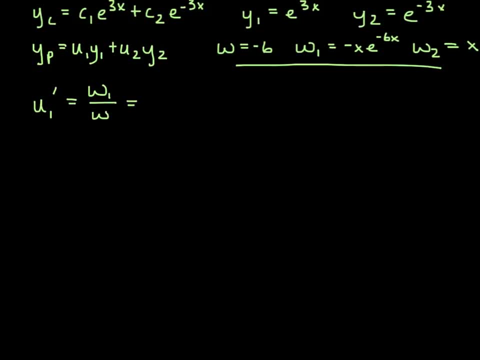 equal w1 over w. In other words negative x, e to the minus, 6x over negative 6.. And then u sub 2 prime. so the derivative of u sub 2 is w2 over w, giving us x over negative 6.. 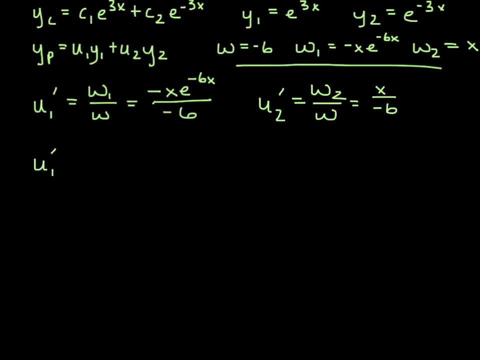 So we'll go ahead and say so: u2.. u sub 1 prime is equal to one-sixth x, e to the minus 6x. u sub 2 prime is just negative one-sixth x. And so to find out what u1 and u2 are, we need to actually integrate. 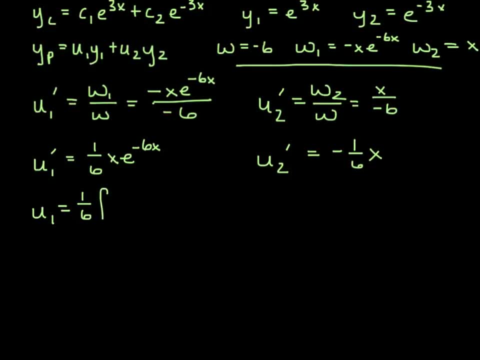 So in other words, u1 is equal to one-sixth integral x, e to the minus 6x dx. u2 is going to be equal to negative one-sixth integral of x, dx, And so the one on the left. here we would do integration by parts. 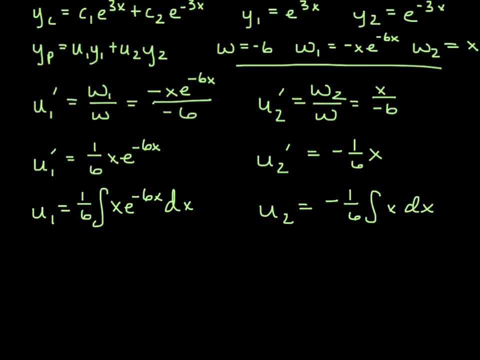 u2, we would just do straight away. So when we figure out u sub 1, we should get negative one over 36 x e to the minus 6x minus 1.. 1 over 216 e to the negative 6x technically plus c. 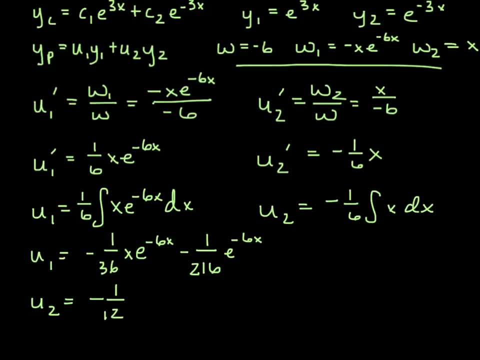 u2, that will be negative 1 over 12 x squared, And so now, just using y sub p equals u1, y1 plus u2, y2,. so that'll be. here's our y1 and our y2.. Here's our u1 and our u2.. 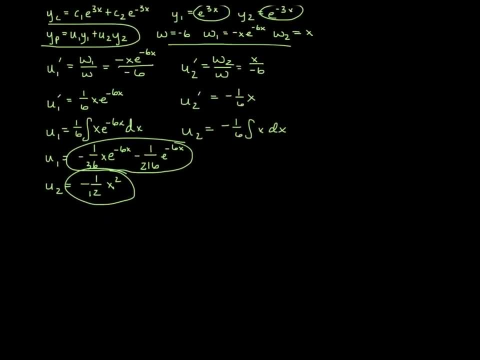 So this tells us y sub p is going to equal u1, so we'll write all that down again. times y1, and y1 was e to the 3x x plus u2.. u2- y2, so we have u2- is negative. one-twelfth x squared, y2 was e to the minus 3x. 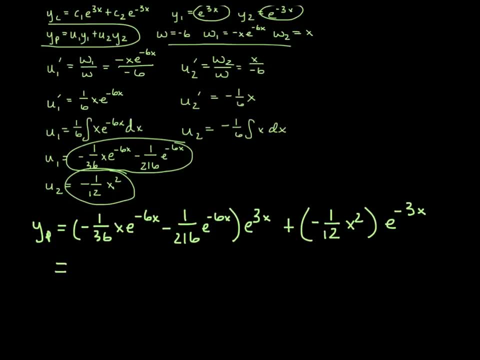 So when we do some simplifying there, that will give us negative 1 over 36 x e to the minus 3x, minus 1 over 216. e to the minus 3x minus One-twelfth x squared e to the minus 3x. 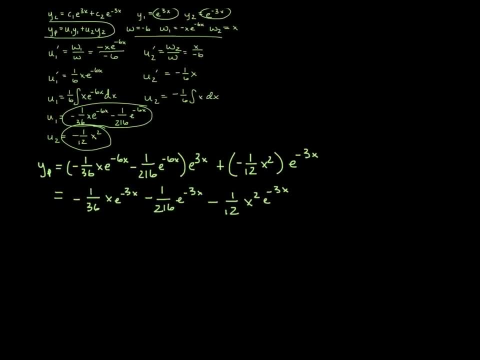 All right, so now we just need to write the solution, And so y is equal to y sub c plus y sub p. So y sub c, we said, was c1, e to the 3x plus c2, e to the minus 3x. 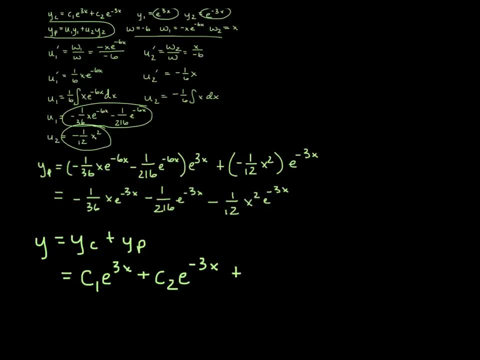 plus c2, e to the minus 3x, And then we'll include the y sub p. So I guess actually we'll go ahead and say: minus 1 over 36 x, e to the minus 3x. minus 1 over 216: e to the minus 3x. minus 1 over 12 x squared, e to the minus 3x. 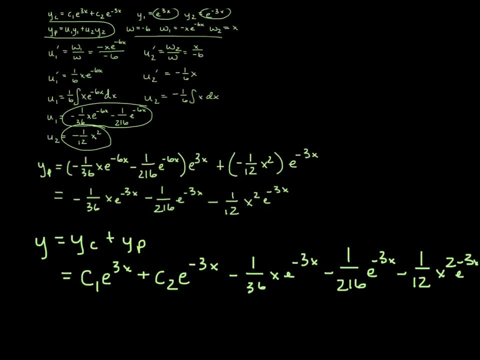 And the thing we want to notice here is that technically our c2 e to the minus 3x is going to be negative 1 over 36 x e to the minus 3x And negative 1 over 216 e to the minus 3x. these are both like terms, right. 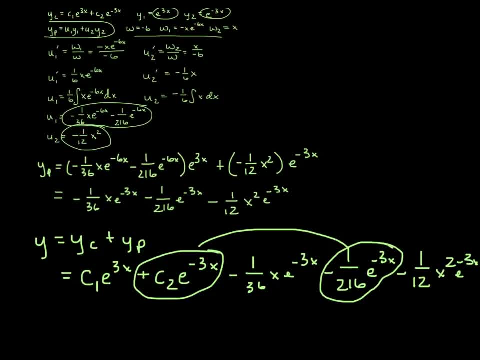 We have an amount of e to the minus 3x, another amount of e to the minus 3x, since we don't know what the constant really is. here We have a constant minus 1 over 216, which is just going to be some unknown constant.